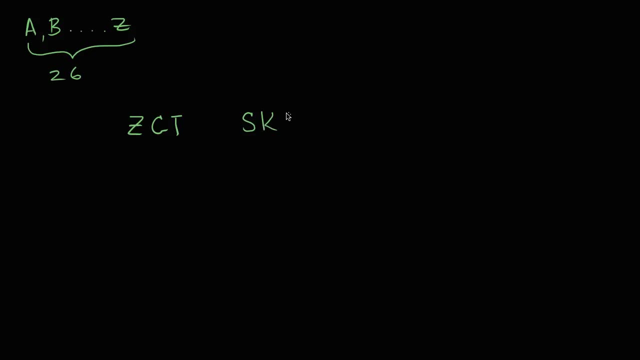 Or the word, the word, the word scudge would be a legitimate word in this example. So how many possible three-letter words are there in the English language? I encourage you to pause the video and try to think about it. All right, I assume you've had a go at it. 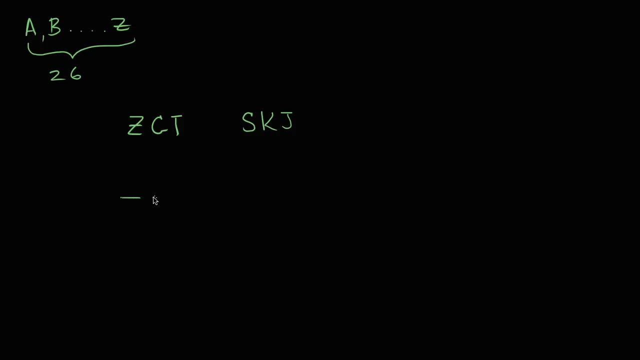 So let's just think about it. For three-letter words, there's three spaces. So how many possibilities are there for the first one? Well, there's 26 possible letters. for the first one, Anything from A to Z would be completely fine. 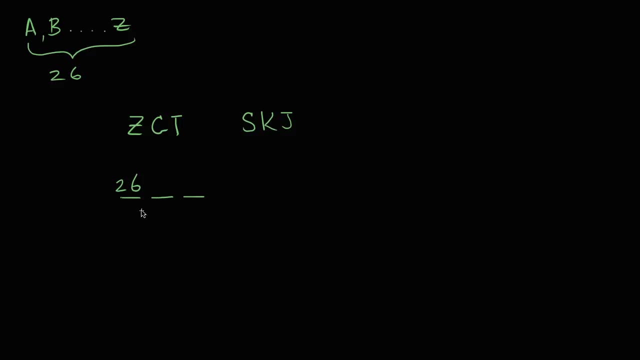 Now, how many possibilities for the second one, And I intentionally ask this to you to be a distractor, because you might be. you know, we've seen a lot of examples where we're saying, oh, there's 26 possibilities for the first one. 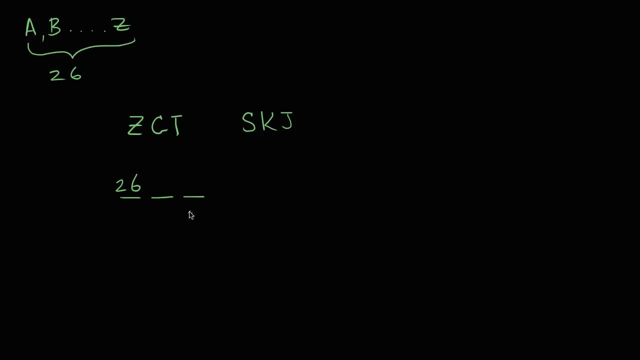 and then maybe there's 25 for the second one and then 24.. And then 24 for the third. But that's not the case right over here, because we can repeat letters. I didn't say that all the letters had to be different. 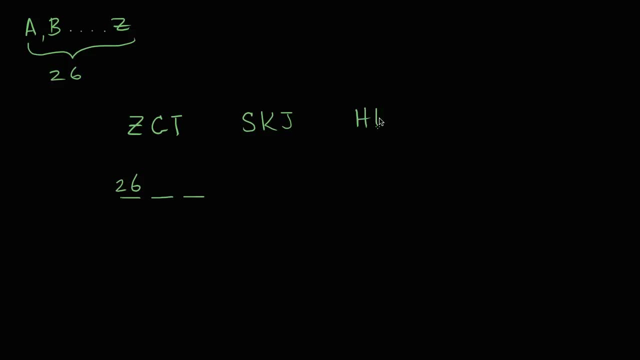 So, for example, the word, the word would also be a legitimate word in our example right over here. So we have 26 possibilities for the second letter and we have 26 possibilities for the third letter. So we're going to have- and I don't know what this is- 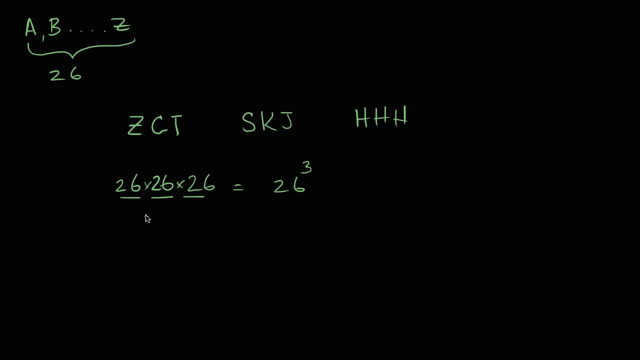 26 to the third power possibilities, or 26 times 26.. And you can figure out what that is. That is, how many possible three letter words we can have for the English language if we didn't care about how pronounceable they are. 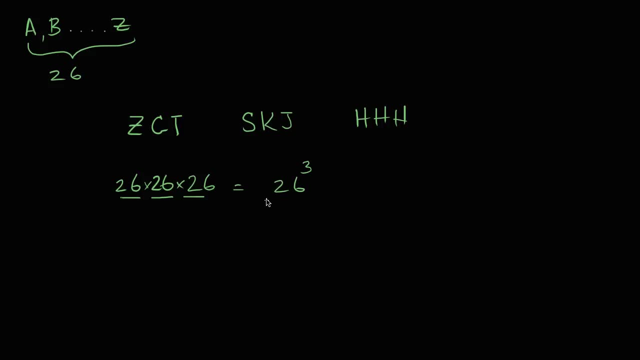 if they meant anything and if we repeated letters. Now let's ask a different question. What if we said how many possible three letter words are there? if we want all different letters, So we want all different letters, So these all have to be different letters. 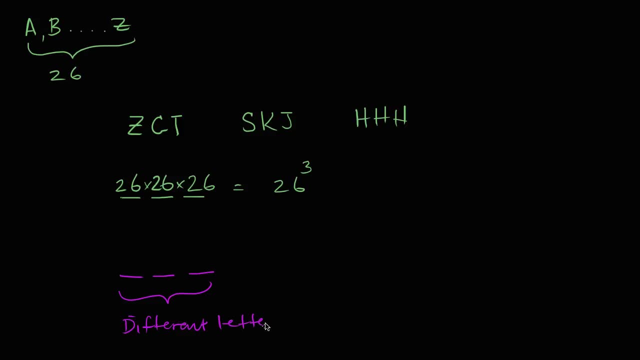 Different, different letters And once again pause the video and see if you can think it through. All right, So this is where permutations start to be useful. Although I, you know, I think a lot of things like this, it's always best to reason through. 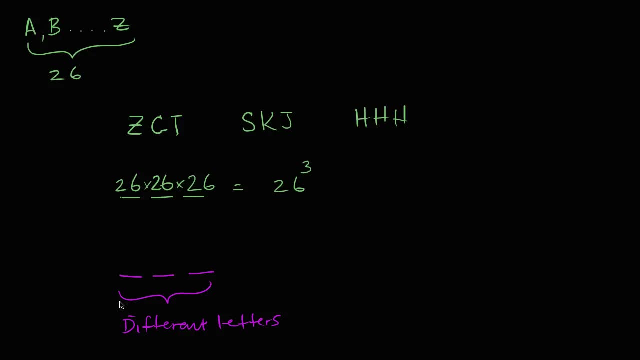 than to try to figure out whether some formula applies to it. So, in this situation, well, if we went in order, we could have 26 different letters for the first one, 26 different possibilities for the first one. You know, I'm always starting with that one. 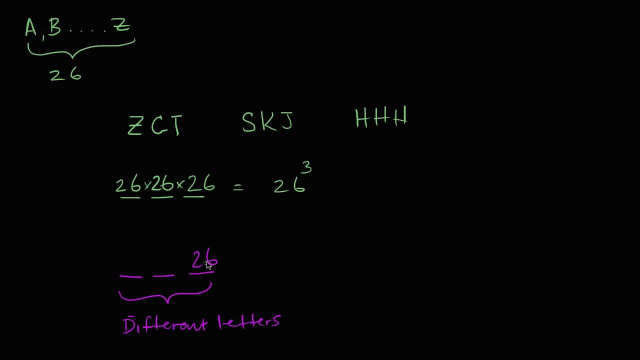 but there's nothing special about the one on the left, We could say that the one on the right. there's 26 possibilities. Well, for each of those possibilities, for each of those 26 possibilities, there might be 25 possibilities for what we put in the middle one. 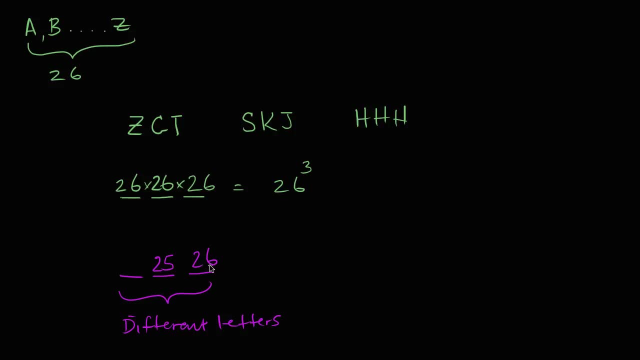 if we say we're going to figure out the middle one next, And then for each of these 25 times 26 possibilities, for where we figured out two of the letters, there's 24 possibilities because we've already used two letters for the last bucket that we haven't filled. 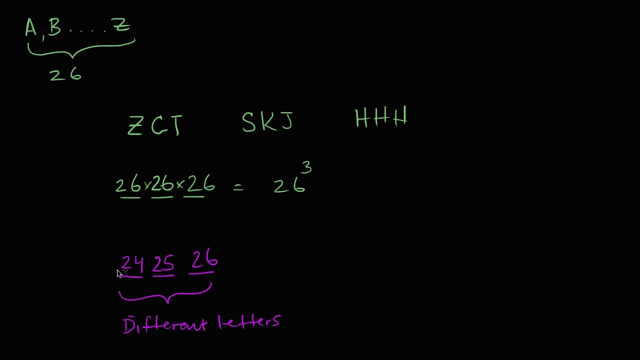 And the only reason why I went 26,, 25,, 24 is to show you there's nothing special about always filling in the leftmost letter or the leftmost chair first. It's just about. well, let's just think in terms of. 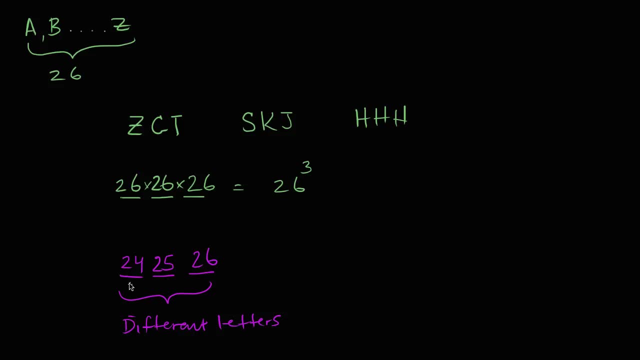 let's fill out one of the buckets first. Hey, we have the most possibilities for that Once we use something up, then for each of those possibilities we'll have one less for the next bucket. And so I could do 24 times, 25 times 26,. 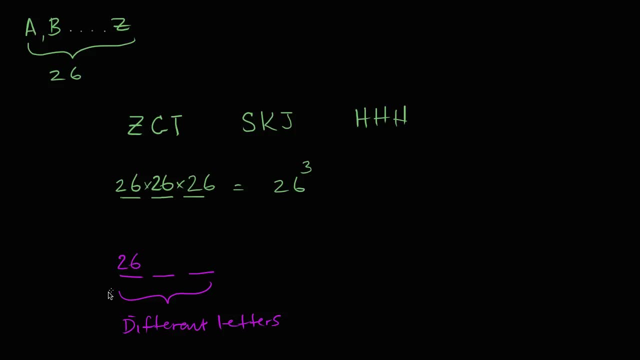 but just so I don't fully confuse you, I'll go back to what I have been doing: 26 possibilities for the leftmost one. For each of those, you would have 25 possibilities for the next one that you're going to try to figure out. 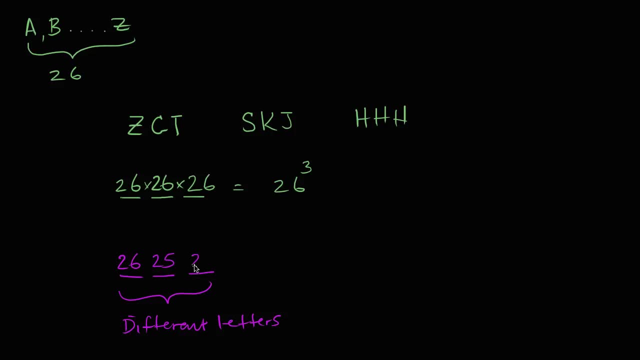 Because you've already used one letter and they have to be different, And then for the last bucket you're going to have 24 possibilities. So this is going to be 26 times 25 times 24, whatever that happens to be. 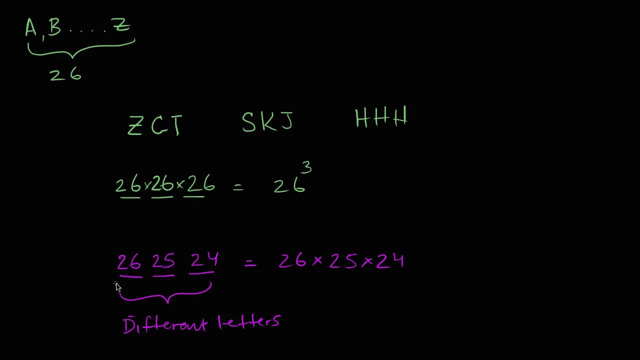 And if we wanted to write it in the notation of permutations, we would say that this is equal to: we're taking 26 things- sorry, not 2p 20,, my brain is malfunctioning- 26,. we're figuring out how many permutations are there? 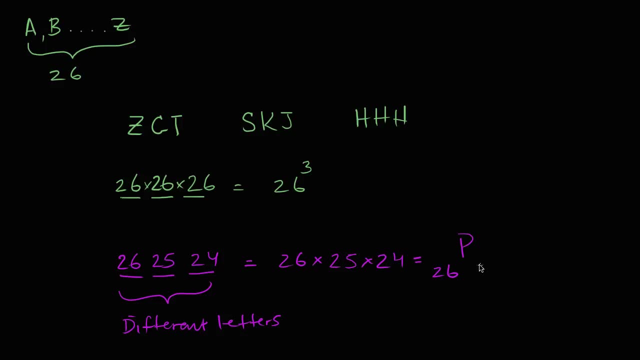 if we're putting 26 things into 3 different spaces, And this is 26,. if we just blindly apply the formula, which I never suggest doing, it would be 26 factorial over 26 minus 3 factorial, which would be 26 factorial over 23 factorial. 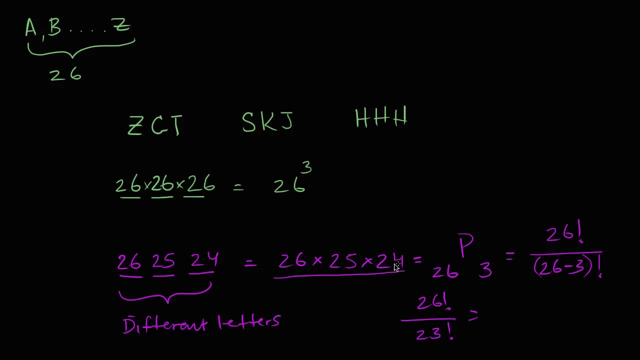 which is going to be exactly this right over here, Because the 23 times 22 times 21, all the way down to 1, is going to cancel with the 23.. And so the whole point of this video. there's two points.